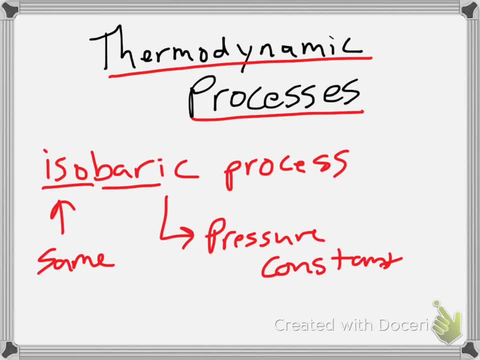 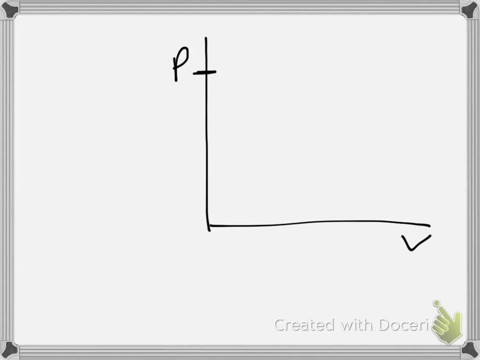 pressure. And if we, When we take a look at what that looks like on a PV diagram or pressure versus volume diagram, we're keeping the same pressure but we're changing the volume. So we could move from point A here to point B over here And that would be an isobaric process And it could actually go either way, right? It? 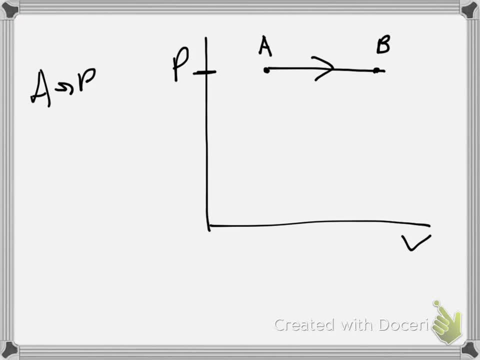 could go from A to B And from A to B. that would be an expansion of volume, And then we'd have a volume, so we would call it an isobaric expansion. but you could also have the exact same thing going from B to A, in which case that would be an isobaric compression. 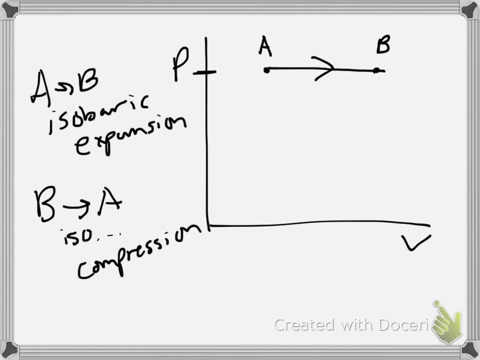 Either way, though, we do know that we do actually have some work happening here, because we saw in class that the work is the area underneath this graph. So the work was the negative pressure times, the change in volume, and that gives you the work for an isobaric process. 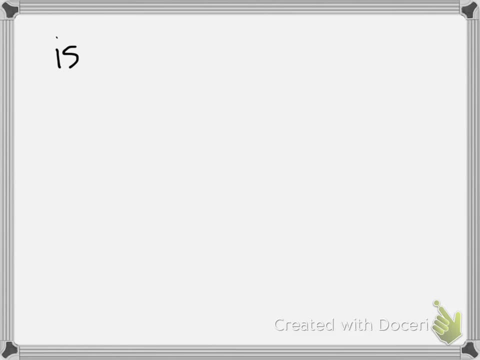 So the next one that we're going to look at is called isochoric- or I'm going to go or- or Isovolumetric. Okay, isochoric or isovolumetric. So again we've seen that iso and the iso means same right. 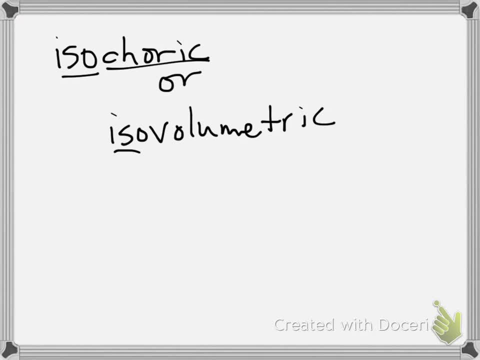 The original one- isochoric is how AP used to refer to this- but now they have this new one that they're liking to use more, and it's isovolumetric. So you can probably see from the secondary term that what we're talking about is the. 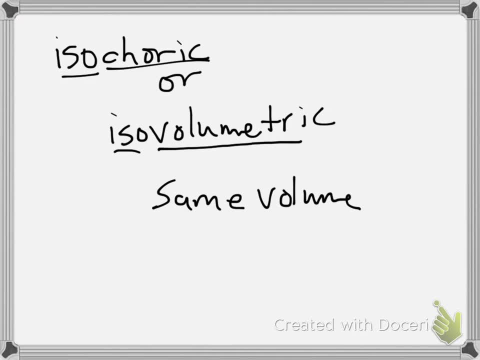 same volume, same volume. So in this one we really don't have that. We don't have an isochoric or an iso or, excuse me, we don't have a compression or an expansion, because we're saying that the volume remains the same. 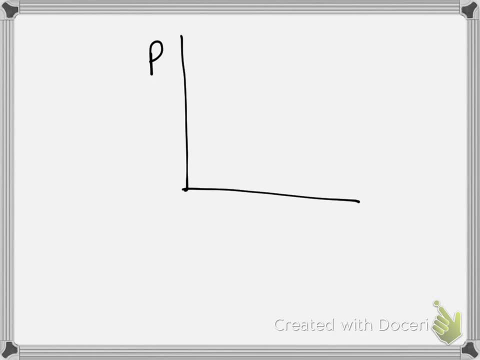 So on a PV diagram- pressure volume- we're talking about having the same volume, So we can have point A here and we could have point B up here, in which case you go from A to B or B to A. It doesn't necessarily matter which way you go, unless you're talking about a certain process. 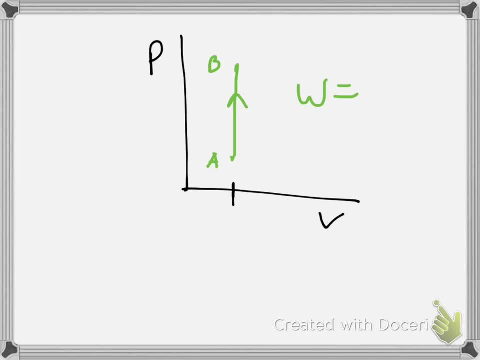 but we don't have any work done here. The work is exactly equal to zero because there's no area underneath that particular line. Now if you were moving from A to B saying the same volume but having an increase in pressure, then we know from what is the one Charles law? I think it is that pressure. 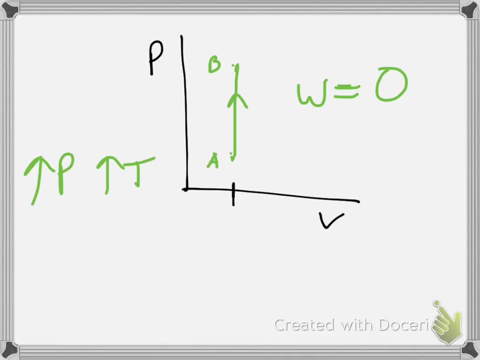 goes up, therefore, temperature has to go up, so that means heat had to have flowed into the system here. If it's the other way around, pressure goes down, That means temperature has to go up. Temperature had to have gone down, which means that we had to take heat out of the. 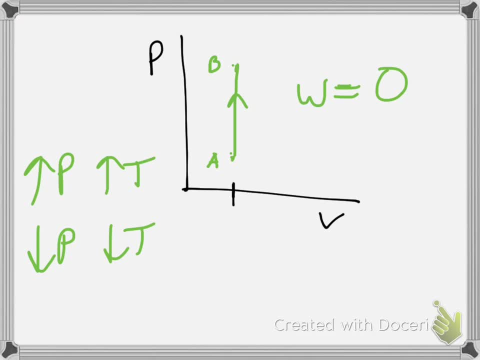 system. We had to remove energy from the system, So it's isochoric or isovolumetric. The next one is called isothermal. Again, we're saying the iso, which means same. You can probably figure out that thermal, what that means. 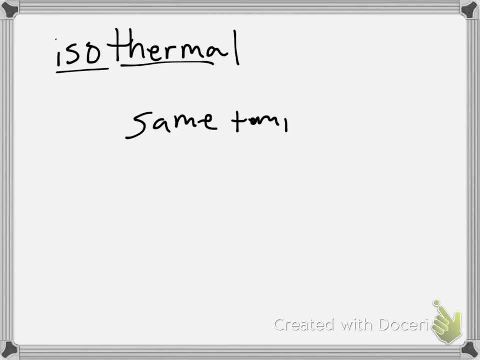 So this is what we're talking about. is the same temperature, The same temperature. Okay, The same temperature, Which means for a given set of gas, so a sample of gas, then what we're talking about is that the same average kinetic energy of the gas and we have to keep the same temperature. 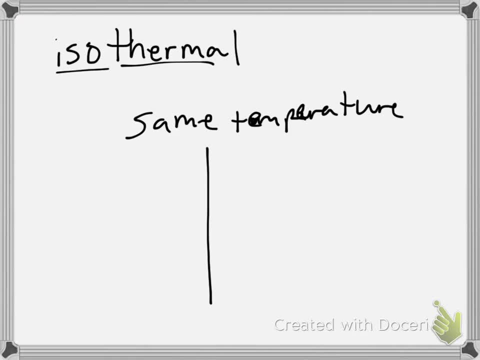 Well, this has got nothing to do with pressure, nothing to do with volume in terms of having to be the same. so that means pressure and volume can actually change. Well, if pressure and volume can change but temperature remains the same, then that means: 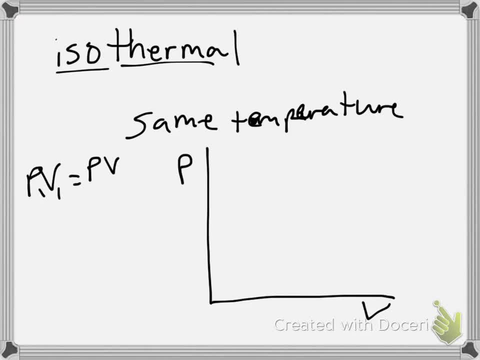 we're actually in a situation of Boyle's law: PV equals PV or P1V1 equals P2V2, and we saw in class that when we plot that pressure versus volume for Boyle's law, then you end up getting this nice curve, this like inverse. 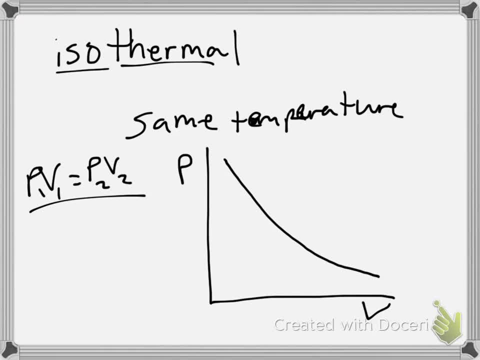 curve kind of thing which makes sense according to this equation right here, that PV would equal a constant, or that pressure would be equal to that number over volume, which would give you an inverse graph like this. The weird thing about it is that 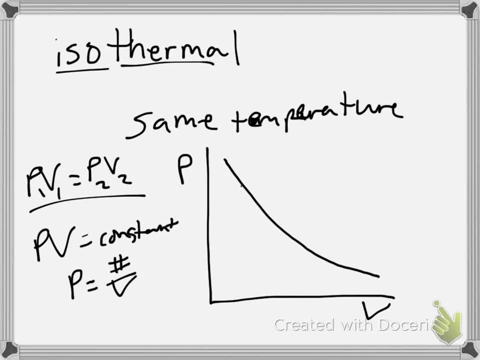 Okay, So every point on this graph, every point on the graph, has the exact same temperature. Every point has the exact same temperature, but we can have a different graph. We could have another graph down here, and because that graph is lower, this would have. 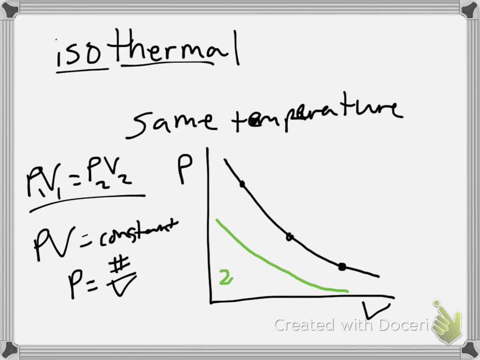 to have a smaller temperature. so this one might be 200 degrees kelvin, but the one up here might be 600 degrees kelvin and the next one might be way up here, and that one could be 1,000 degrees kelvin. 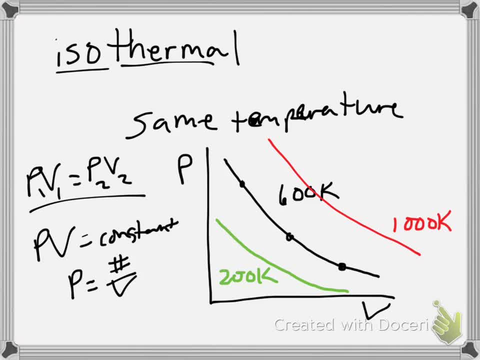 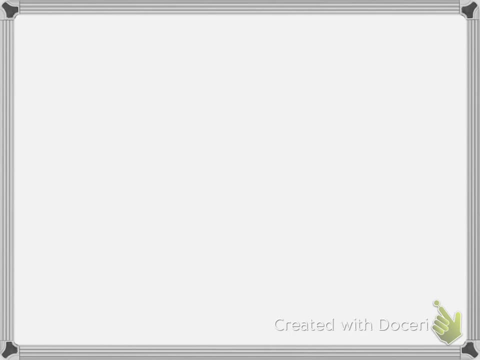 So they're all inverse curves here, but every point on that curve. so, moving from point A to point C and going through point B, each one of these points all has the exact same temperature but has a different pressure and volume. Now work is done on a pressure versus volume graph for an isothermal situation. okay, but 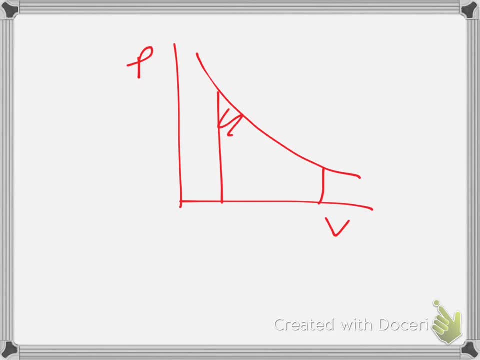 since we have an inverse curve here, you would need to know a little bit of calculus in order to figure out that You could estimate it. You could, you know, make a rectangle and a triangle or something like that, but you'd need a little bit of calculus in order to actually find the work here. 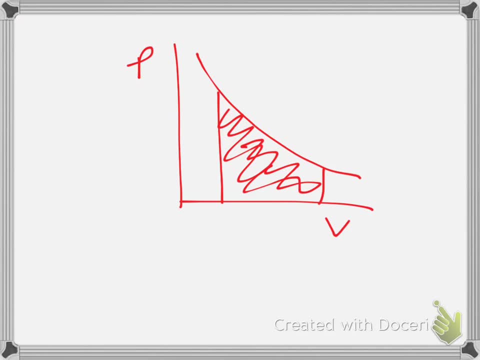 So if we're keeping the same temperature but our pressure and volume are actually changing, if we're going from point A up here and we're going to point B down here, that means we've increased our volume, so that means we can have an expansion here again. 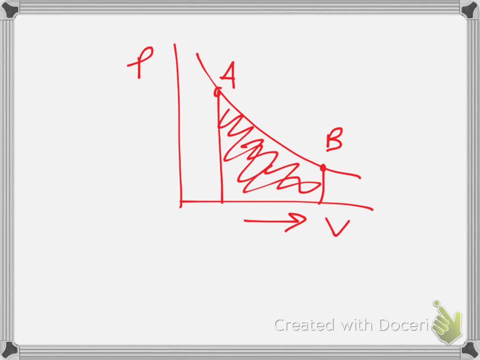 So this is an isothermal expansion. but pressure goes down, volume goes up, temperature remains constant. Now here's the kicker here: If temperature remains constant, pressure is going down, volume is going up. that means that we have to end up actually producing or giving this system heat. so we have to. 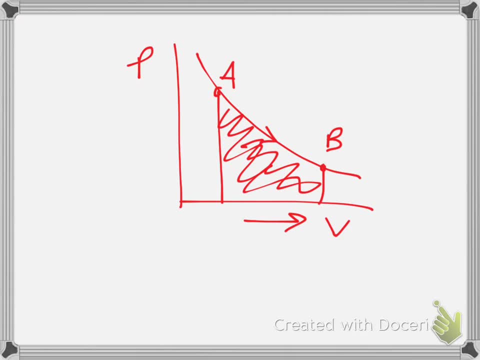 increase the amount of heat going into the system before this compression, excuse me this expansion, in order to keep the temperature constant, in order to keep the molecules moving around with the same average kinetic energy. Okay, true, if we're going back the other way, If we wanted to keep the same temperature, pressure's. 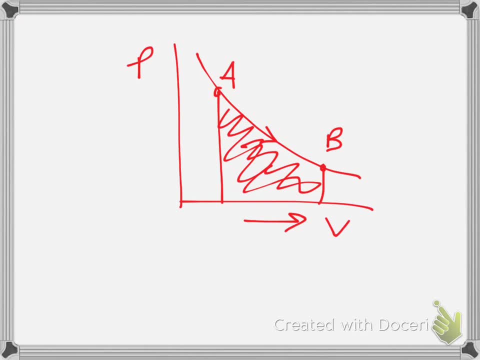 going up, volume's going down, then you end up with having to take heat out of the system. All right. And the last one doesn't follow the same naming conventions. It's called an adiabatic, Adiabatic, And again, we can have an adiabatic expansion or we can have an adiabatic. 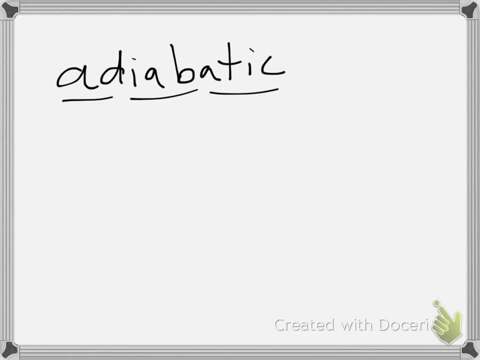 compression. You really can't pick out anything in the word that says what it's actually going to mean. So an adiabatic expansion or compression happens with absolutely no heat lost or gained. So we have the same amount of heat, Or a better way of putting it would be: same amount of. 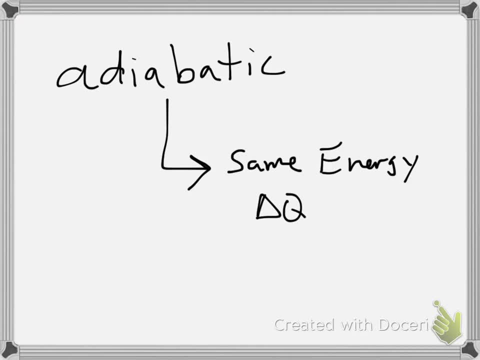 energy. So our Q right heat didn't change, Or we can say: our changes didn't change. Change in Q is equal to zero. Now, this does not mean that pressure remains constant, volume remains constant or even temperature remains constant If something happens like inside. 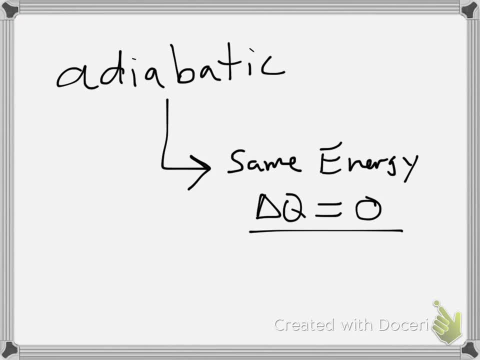 the motors that were taken apart. if the gas expands and it pushes on the piston, then work is being done, in which case volume is going to increase, pressure might decrease, temperature might increase or decrease, depending on what's going on, But we're doing it, so 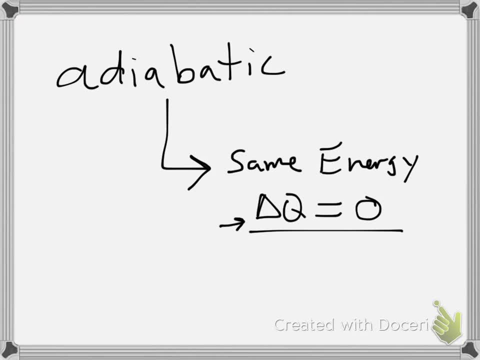 quickly that we're not going to be able to do anything, So we're going to have to do something. We're not allowing any heat to enter or exit from the system. So the way that this looks on a pressure versus volume diagram, because we're allowing temperature. 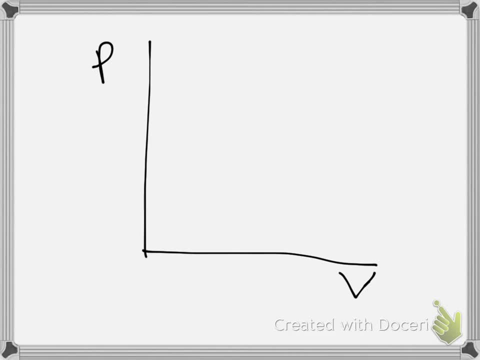 to change. here it actually works as if we were going between two different isothermal lines. So here is our first isothermal line that says maybe this one's at 600 degrees Kelvin, And then here is our second isothermal line. These are inverse ones that are always the same distance away from each other, So maybe 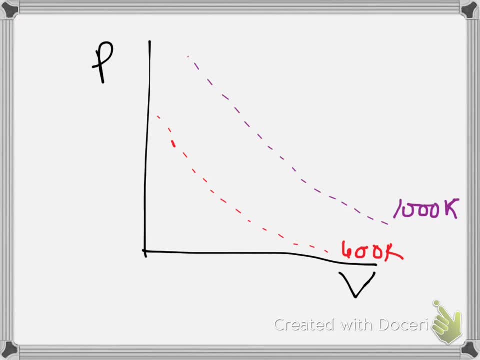 this one is 1,000 degrees Kelvin. Well, if we are looking to get from point A, which is at 1,000 degrees Kelvin, and go to point B, which is at 600 degrees Kelvin, then we're going to need a line that goes kind of curves downward like this, but it's a much steeper. 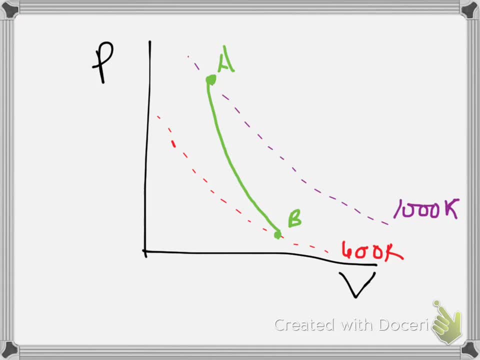 line than what we have for an isothermal line. So this right here from A to B, would be an adiabatic expansion, because we are actually going further in volume, or increasing volume. Again, you go from B to A and it could be an adiabatic compression.